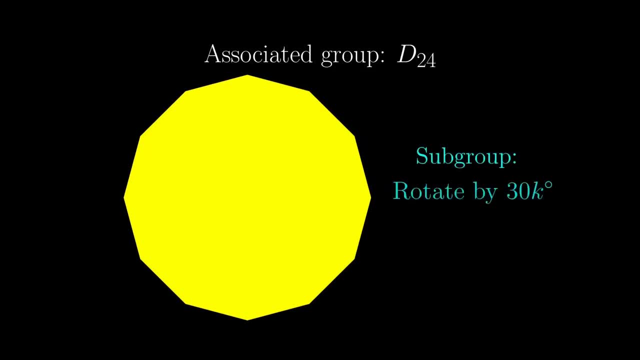 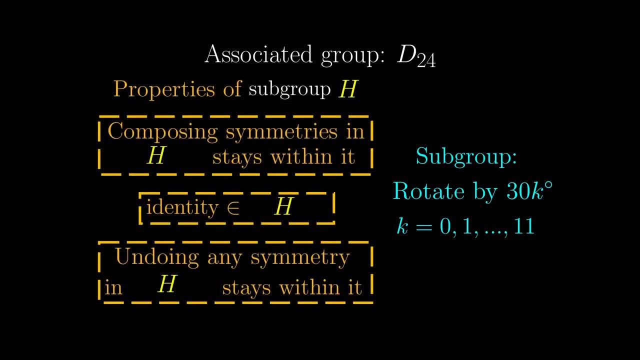 This means we are only considering rotations in either direction by a multiple of 30 degrees. You can use this checklist introduced in the Lagrange's theorem video to check that it 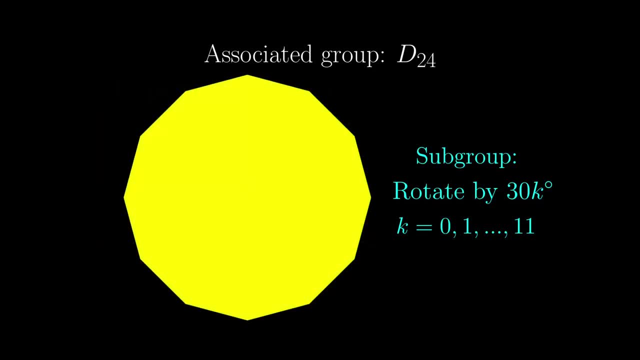 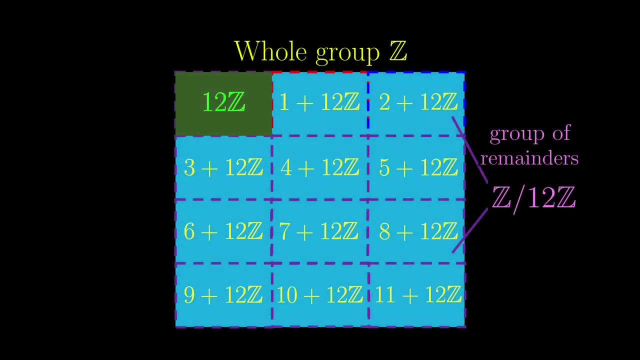 is indeed a subgroup. We temporarily call this group R-12, R for rotation. However, it seems similar to the quotient group Z mod 12Z. We will see why they are similar in a minute. Just a reminder that Z mod 12Z is a quotient group, that is, a group of cosets 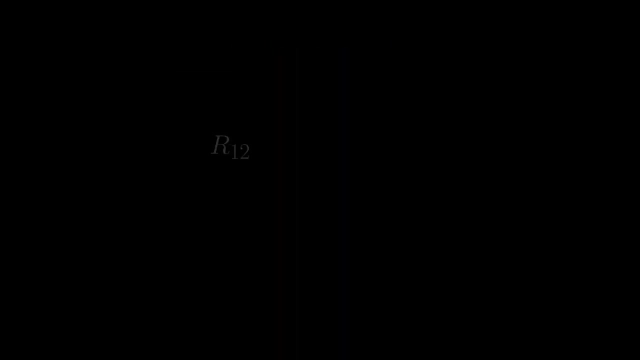 which themselves contain symmetries. So on one hand, we have R-12 with symmetry, and on the other hand, we have R-12 with symmetry. 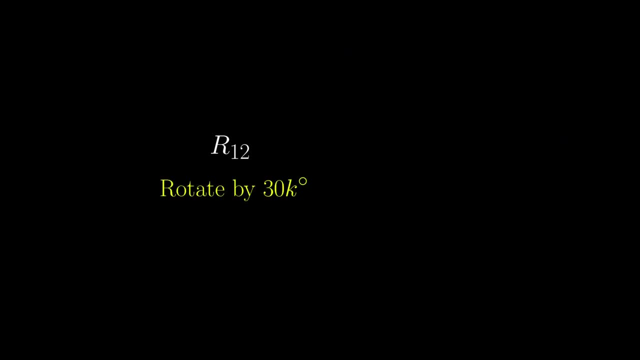 We have Z mod 12Z, which is a group of cosets of 12Z written this way. It's tempting to say that these two groups are the same, but R-12 is fundamentally a group consisting of rotational symmetries of the dodecagon, while Z mod 12Z is fundamentally a group consisting of cosets of the dodecagon. 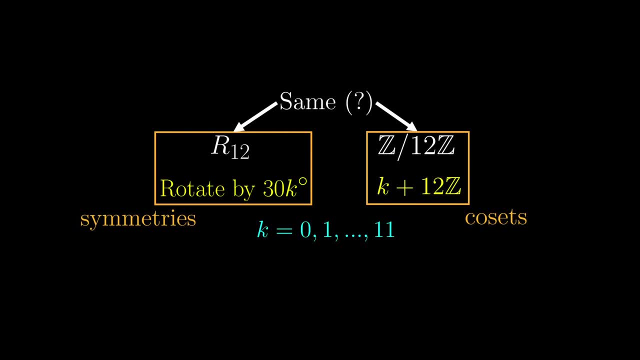 possibile of homomorphism & isomorphism. 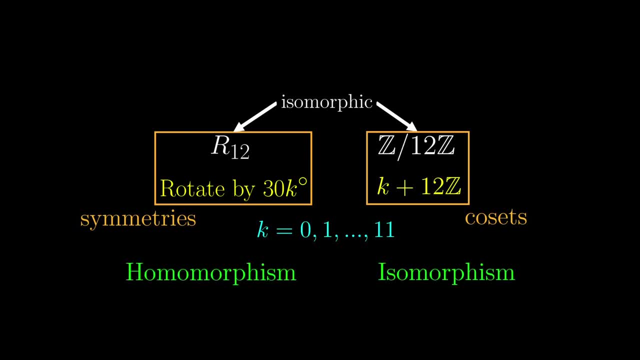 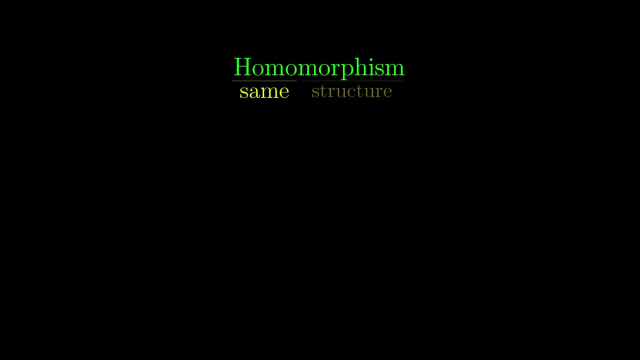 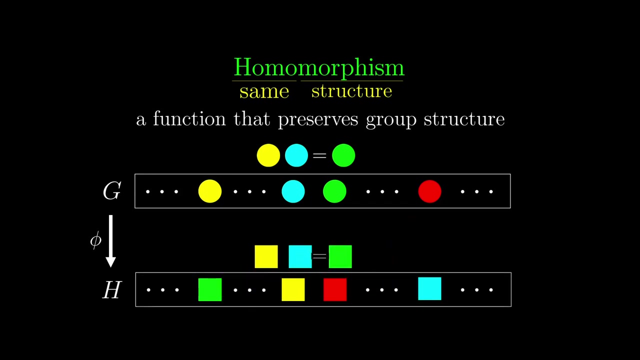 This video deals with the concept of homomorphisms and isomorphisms, which is strange in terms of naming because both homo and iso mean sane, but isomorphism is a stronger kind of sane than homomorphism. Let's start with homomorphism. As said before, homo means same, and morphism here could mean the group structure. Roughly speaking, it is a function from a group to another that preserves the group structure. Let's say we have a group G, which can be illustrated more colourfully as such, where each blob represents an element in G. Suppose that in the group G, when we concatenate yellow and blue blobs in this particular order, we get a green blob. Let's say there is a function phi from G to another group H, and it maps these circles to squares in the group H. Now if we concatenate yellow square and blue square in the exact 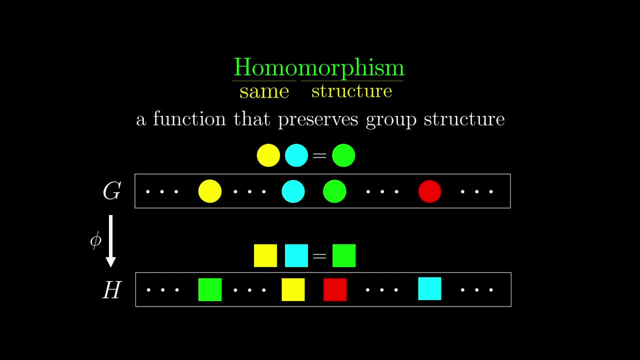 same order as before, we might get the green square. If, for every possible relation that you have for the group G, you have the correct corresponding relation for group H, then this function phi is called a homomorphism from G to H. 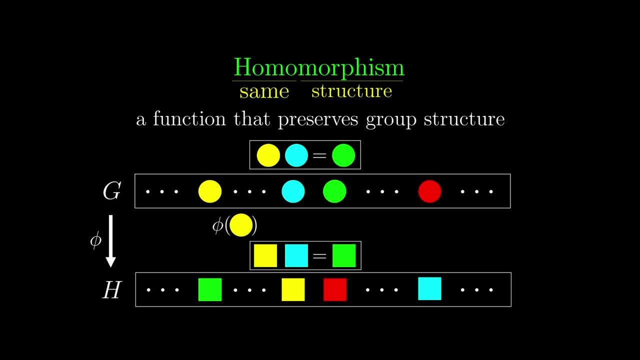 To put it more succinctly, the yellow square is actually the image of the yellow circle under the map phi. Similarly for the blue square and the green one. However, because 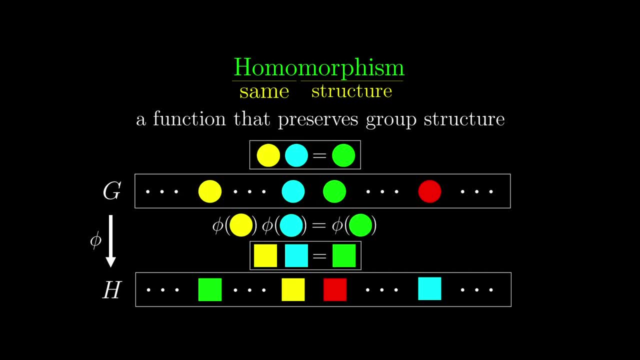 of how yellow, blue and green circle are related to each other, we can replace the green circle with this. Basically, if this relation holds for all pairs of elements in the group G, then phi is a homomorphism. This is what you will see in a textbook, of course with symbols, not these circles. Now this 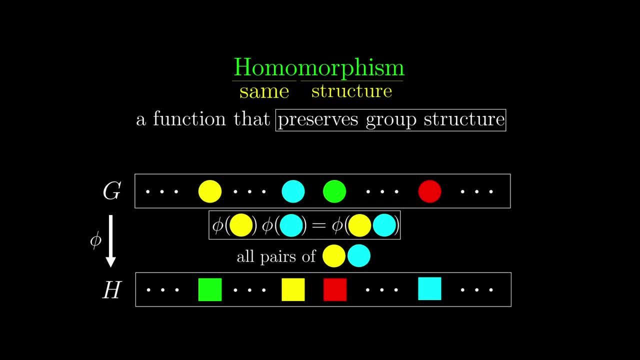 function phi preserves group structure in the sense that all the compositions of symmetries remain intact through this map. 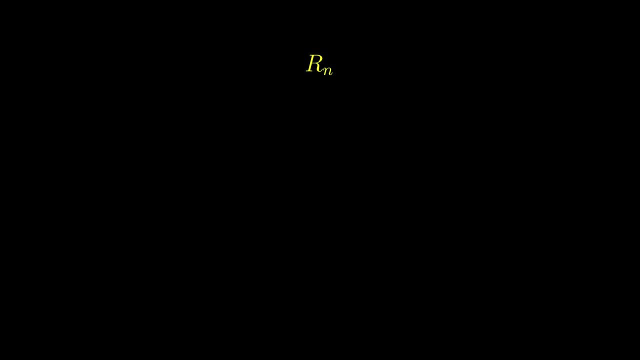 Now, we are going to see an example of a kind of unexpected homomorphism, first by denoting Rn as the group of rotational symmetries of a regular n-gon, generalising the case when n equals 12 that we discussed. It turns out that we can actually construct a homomorphism from R8 to R4, which is pretty unexpected considering that they have different numbers of symmetries. 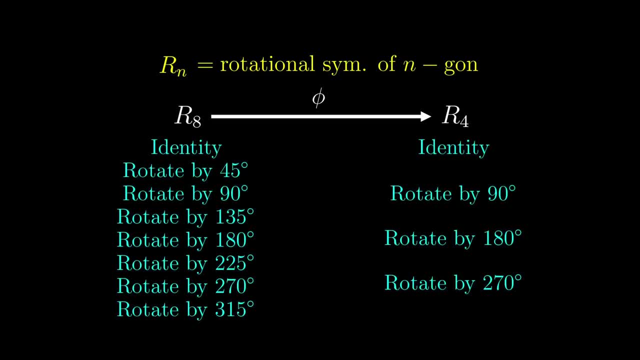 Let's list all the symmetries in each group. The function maps the symmetries like what's shown here. Just to convince you that this is indeed a homomorphism, we consider this particular pair of symmetries. The result of these two symmetries should be a rotation by 225 degrees. Now apply the function phi to all the symmetries involved. We can verify that the result of the 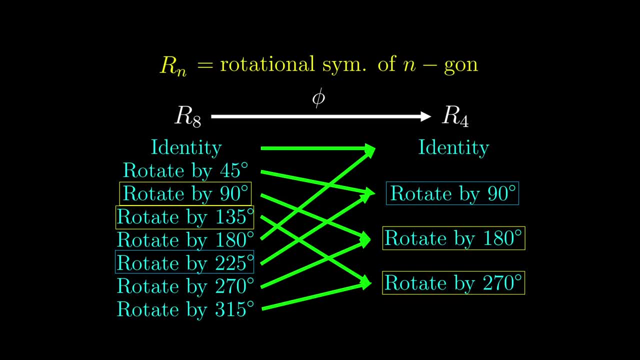 two yellow symmetries on the right does give us the blue symmetry, because a combination of 180 degree and 270 degree rotations does give a 90 degree rotation. But we definitely don't want to say these two groups are the same. The main obstacle is that the function phi is not invertible. If you don't know what that means, this homomorphism phi is not a 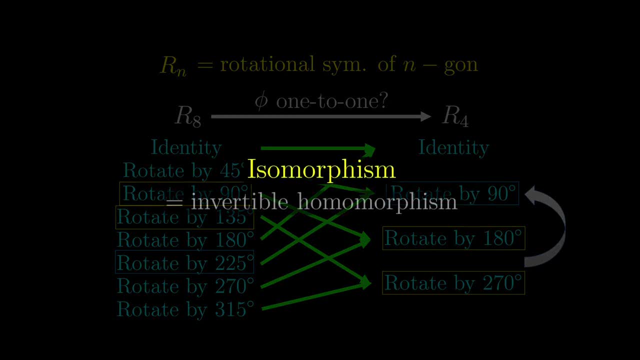 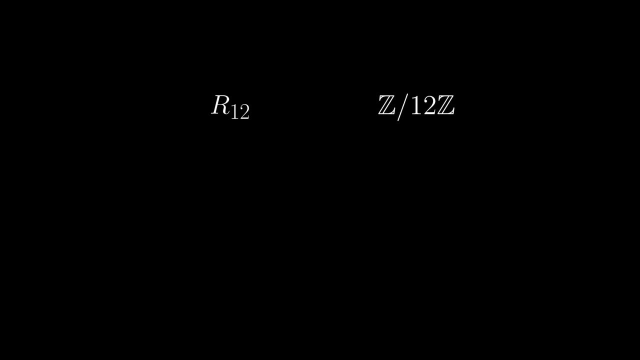 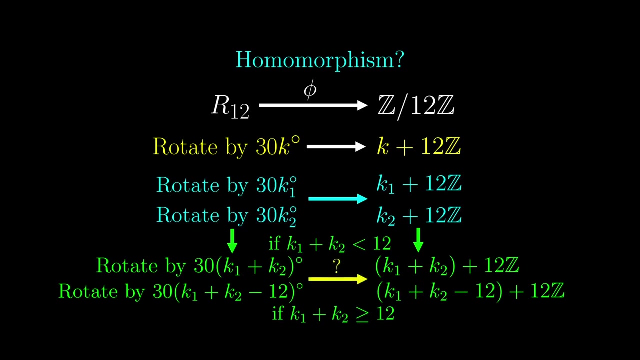 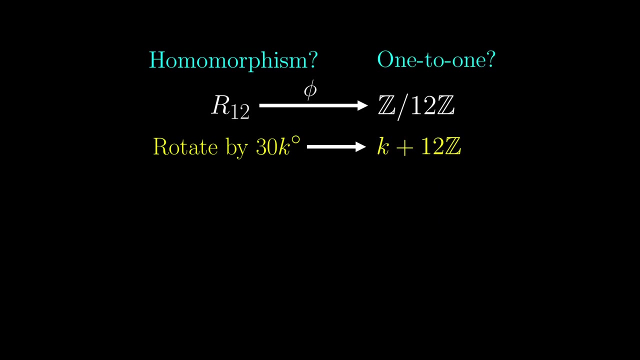 one-to-one function. In fact, any invertible homomorphism is called an isomorphism. To see an example of isomorphism, let's go back to our example at the very beginning of this video. An obvious way to construct an isomorphism phi is to map the rotational symmetry by 30k degrees to the coset k plus 12 z. To check that this is really an isomorphism, we need to first check that it is a homomorphism. We take an arbitrary pair of symmetries on the left, and then map it to something in the quotient group according to the rule described. We then compose symmetries on the left, and compose the cosets on the right separately. Then, we really have to check that the symmetry on the left does map to the coset on the right, under the function phi. If we want to compute the cube symmetry, we'll simply write in the phi. If that is true, then this function phi is a homomorphism. However, we also need to check that it is 1 to 1 in order to say it is an isomorphism. This is obviously true in this case. So this function phi is actually an isomorphism. 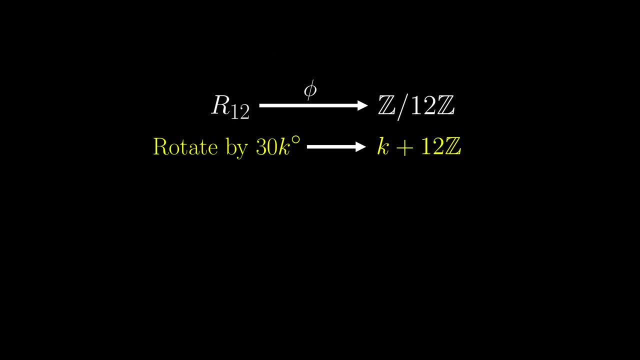 However, this is not the only isomorphism that you can have. For example, this similar looking function is also an isomorphism. This notation here is not really a standard one, but it means the remainder of 5k when divided by 12. You should check that this function is a homomorphism as well as a 1 to 1 function in order to show it is an isomorphism. The difficult part is to show that this function psi is 1 to 1, but we will skip this for this video. 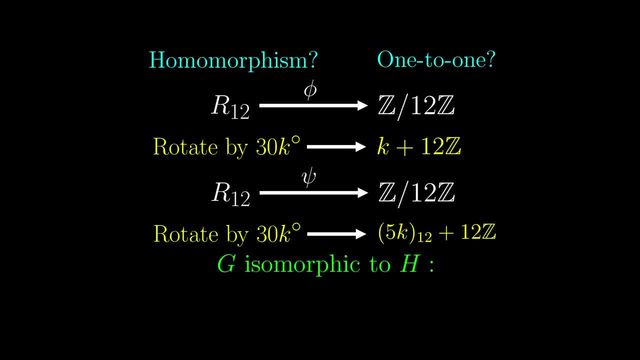 In general, we say the group G is isomorphic to another group H if there is one isomorphism between the groups. We have already shown that the isomorphism might not be unique, but as long as there is an isomorphism, we will call these two groups isomorphic. So since there is at least one isomorphism between R12 and Z mod 12Z, we say these two groups are isomorphic to each other. 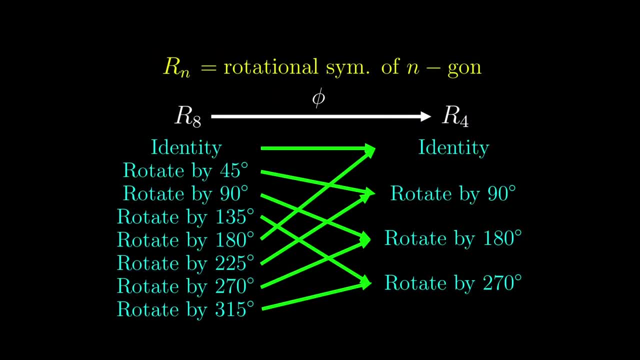 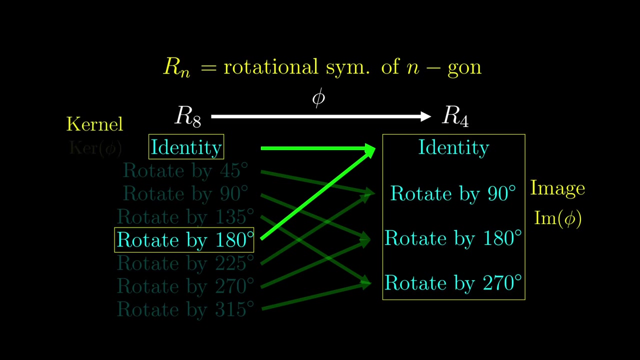 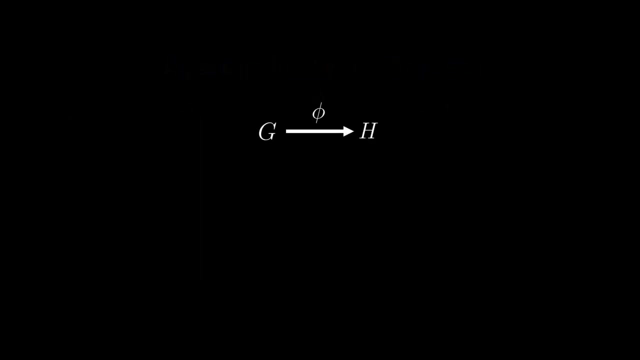 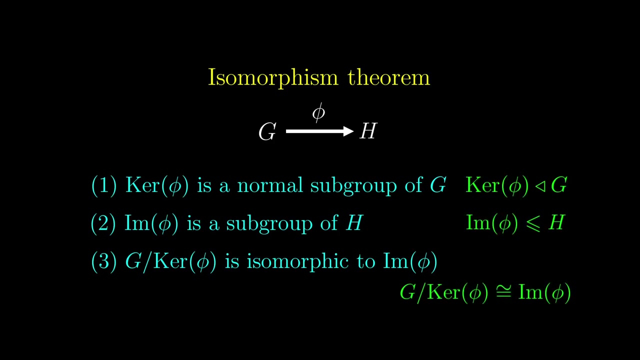 Let's revisit this homomorphism again. As with all functions, we can define the image of this function phi which is something that is hit by the function. This is usually denoted as M of phi. Another thing we are interested in is what symmetries on the left get mapped to the identity on the right. In this case, there are two symmetries. This set of symmetries is called the kernel, denoted as Kerr of phi. We can also define the kernel and image in a general homomorphism. The isomorphism theorem states three things. Firstly, the kernel is a normal subgroup of G. Secondly, we have the image to be a subgroup of H. Lastly, since kernel is a normal subgroup of G, we can define the quotient group. And this quote quotient group is isomorphic to the image. Mathematicians like to use symbols to denote all these concepts, listed on the right here. 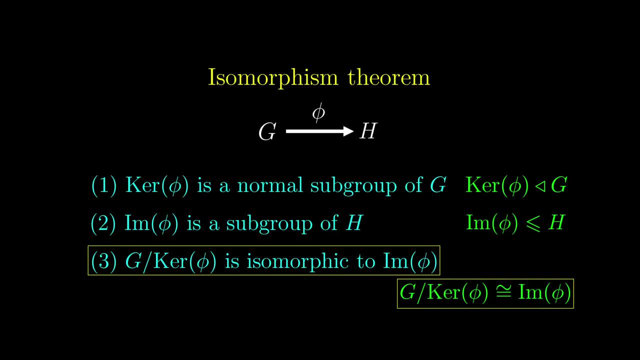 The third statement is what most people think about when it comes to the isomorphism theorem, 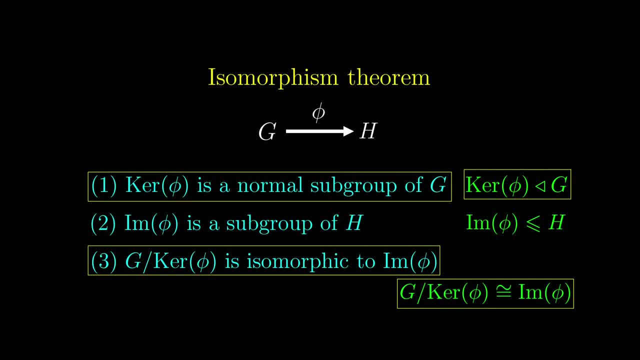 but the first statement is often glossed over, and actually pretty useful sometimes. Proving 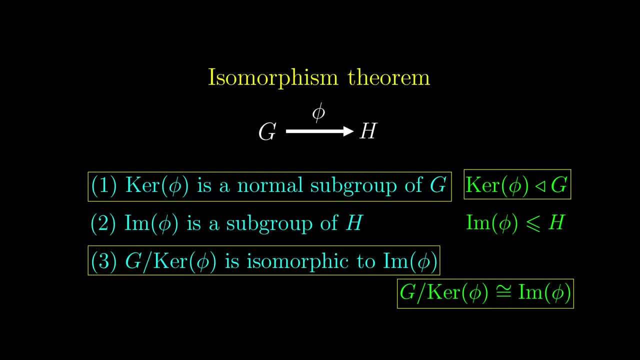 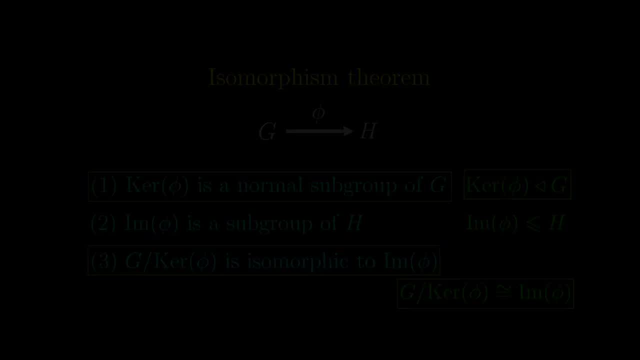 these three statements is not super difficult, but the focus of the rest of this video will be about how we can intuitively understand them. 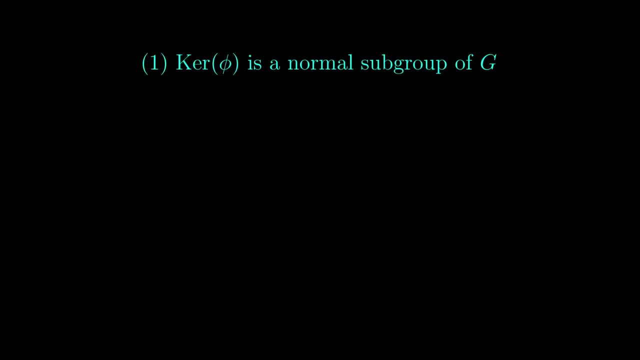 The first statement can be understood as follows. By definition, the kernel is the set of all symmetries that gets mapped to the identity of the other group. As a result, the kernel actually acts like the identity, which looks the same in all possible positions. 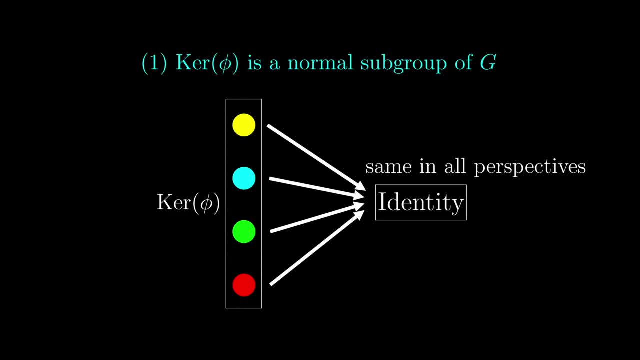 So intuitively, we can see why the kernel is a normal subgroup. If we really need to prove the second statement here, we will need a subgroup checklist. However, 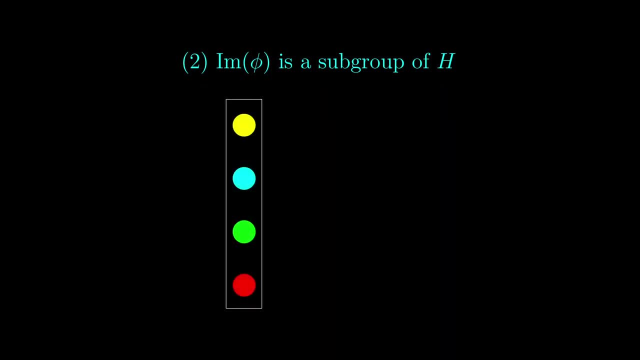 we can use the type of thinking as before. The whole group G is mapped to the image by definition of the image. So the image acts like the entire group G itself. Of course, the image is a subset of the group H, and because it is a group, it is a subgroup of the entire group H. 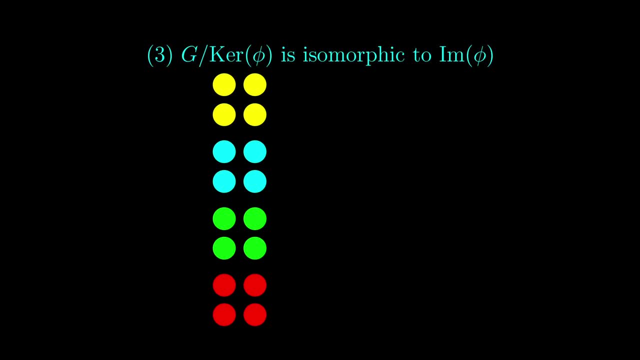 Now what about this third statement? Let's say this is the entire group, and this subset is the kernel of the homomorphism. And these are the cosets of the kernel within the group G. And consider the image of the homomorphism. Let's say this yellow square represents the identity in the image. Then, by definition of the kernel, it gets mapped to the yellow square. It is not too wild to assume that all the symmetries in the same coset gets mapped to the same thing in the image. So one coset can get mapped to one symmetry in the image, and hence, these two groups are isomorphic. Now of course, all these are just intuitive understanding of the theorem. 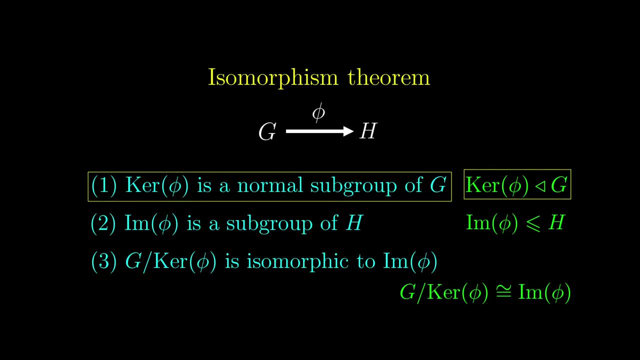 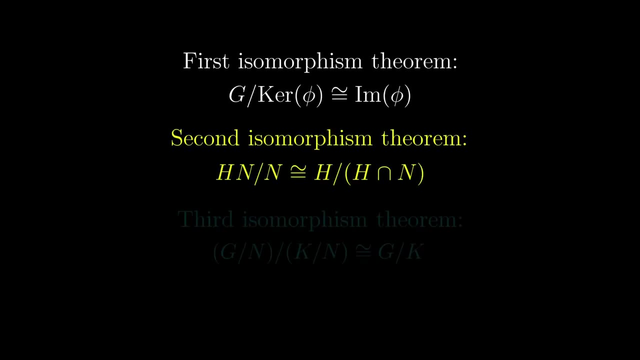 Not a rigorous proof. As a side note, the reason why the first statement is important is that it offers a way to prove something is a normal subgroup easily. This is sometimes also called the first isomorphism theorem, because there are second and third isomorphism theorems. However, all these theorems can be derived from the first one, using clever choices of the homomorphism phi. 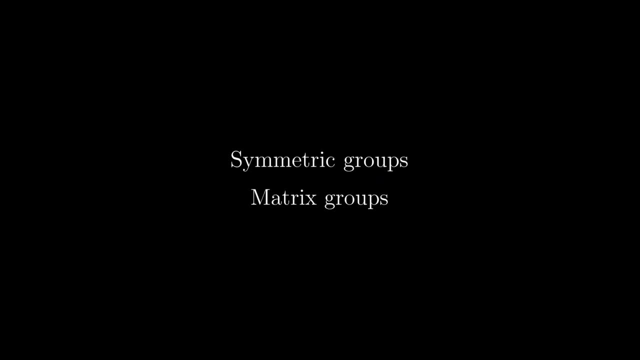 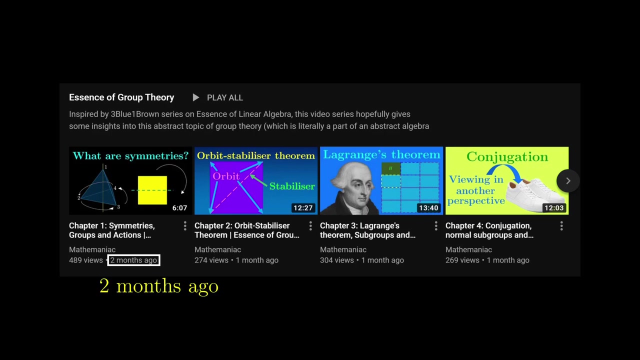 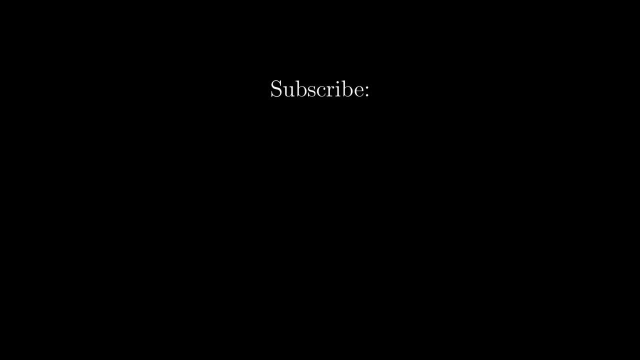 In a formal course on group theory, you might spend a great deal of time on symmetric and matrix groups. But I will not cover those topics, because most concepts will be specific to those types of groups, and not applicable in general. And this is also because this video series has already been up for so long that I am not sure whether viewers like you are bored with it. That does not mean group theory will not be on this channel anymore, because I might talk about some interesting applications, but it highly depends on your enthusiasm towards the idea. If you enjoyed this video series or find it useful, like and share it. Don't forget to subscribe with notifications on. See you next time! Subtitles by the Amara.org community 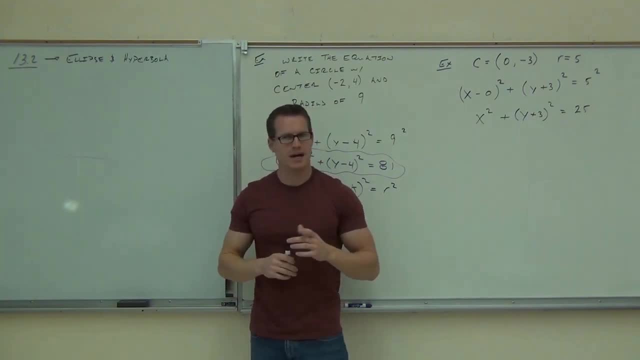 Now, there are a couple other shapes, one of which you might have seen before. The other one, I guarantee you haven't. We're going to talk about, in section 13.2, ellipses and a hyperbola. 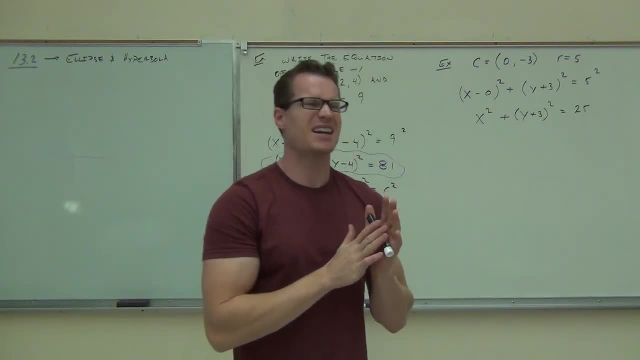 Now, an ellipse is kind of like a circle, but it's not exactly a circle. You ever go to the gym and you see those big, round, like, they're usually blue or gray, those exercise balls? And they're pretty much, it's a sphere, actually, but if you look at it from the profile, it's a circle, right? Now, I'm a pretty big guy. If I sit on one of those circles, is it still going to be a circle? No, it's going to go, right? And it's going to kind of smush out the sides. Well, it's going to have, like, a shape in the middle, but ignore that. So, and it's going to be completely flat on the bottom. 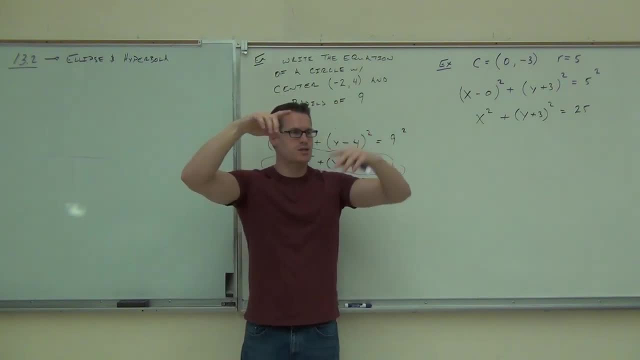 But if you ignore the completely flat part, it looks kind of like an ellipse. An ellipse looks very much like a squished circle. It's what would happen if you took your cone, remember those cones we had? And you didn't slice it straight across, you sliced it diagonal. You're not going to get a circle, you're going to get an ellipse. It's an elongated circle. That's where we get this ellipse from. So an ellipse looks a lot like an elongated circle. So we'll talk about that one first. So here's an ellipse that's centered around . 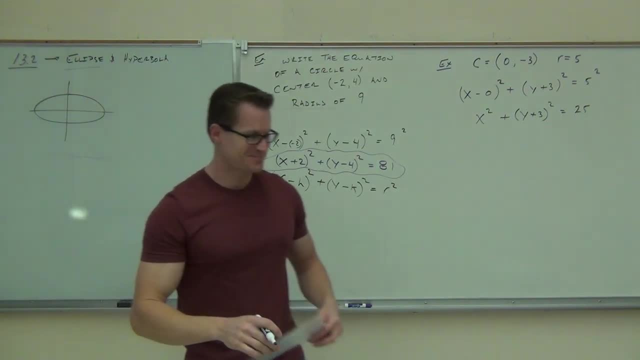 These are my stewy heads, and I've missed my marks.